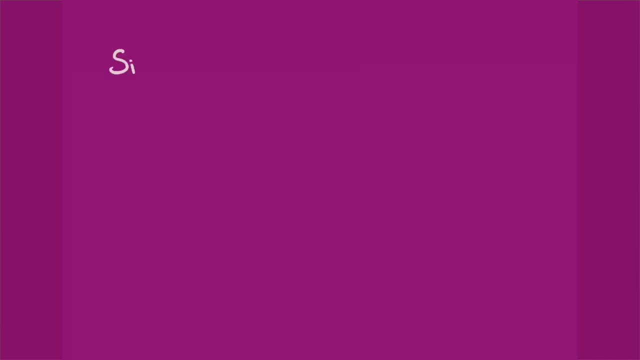 After 140 years of being colonized, Singapore gained its independence in the year 1965. During this time, it was a country with hardly any natural resources to bank on, and the education system, too, had absolutely no uniformity. It was then Prime Minister Lee Kuan Yew's vision that led the country to 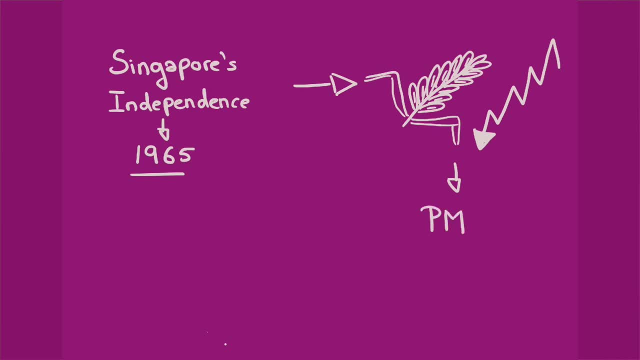 what it is today. He had only one strategy in mind: To invest and develop the country's only natural resource, the people of Singapore, and for this he prioritized the rebuilding of schools. because of the diversity in ethnicities and religions in the country, the schools then operated in different languages, like English. 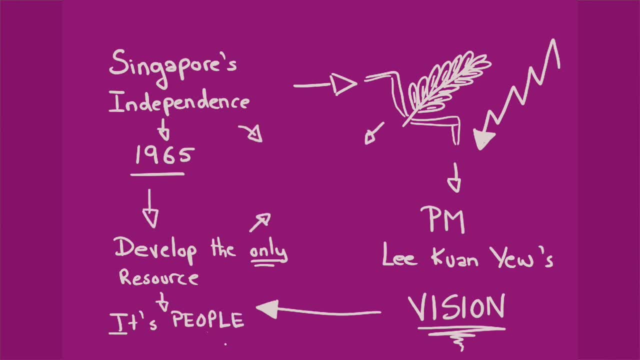 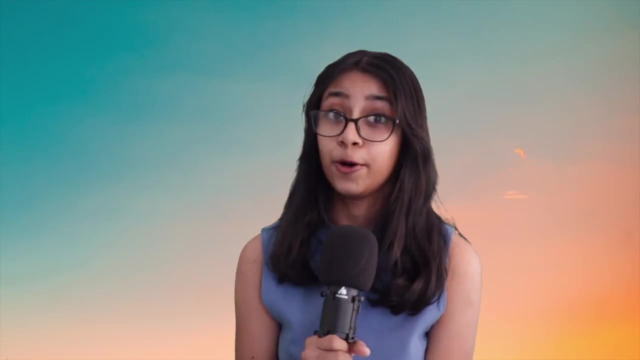 Malay, Chinese, etc. but PM Lee Kuan Yew wanted to encourage social unity among the population, to support economic development and put 20% of the government expenditure in just education. so now let's get into the nitty-gritties and the different aspects about what makes Singapore's education. 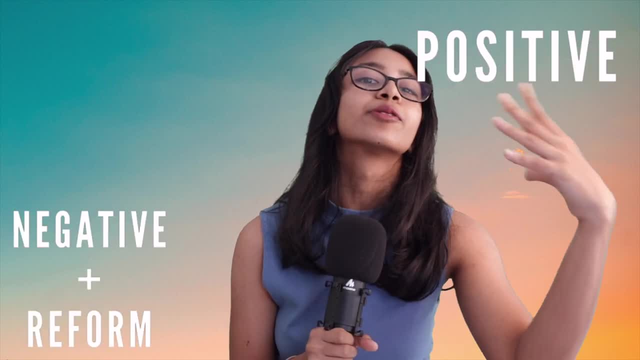 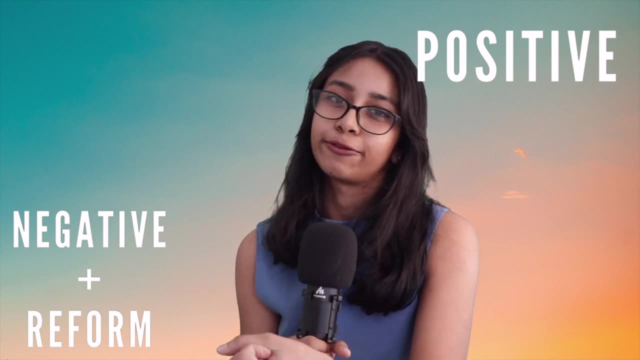 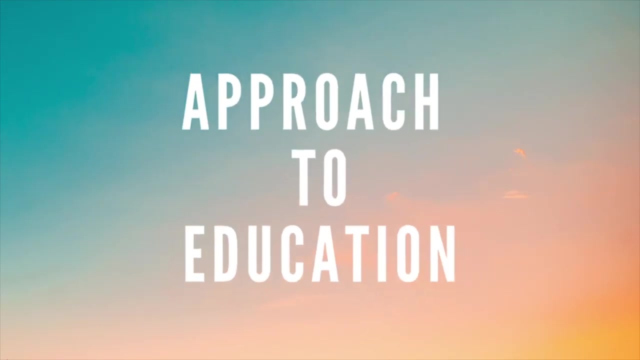 system so special. first let's start with the positives and all the rosy things, and then let's get into the negative and what really needs reform, because, let's be honest, nothing's really perfect right. so let's get into it. schools in Singapore actually believe in using a playful approach when it comes. 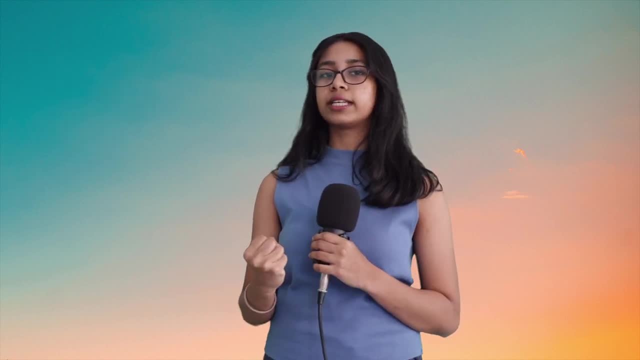 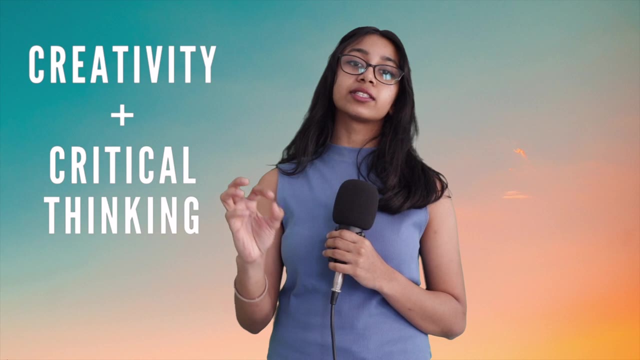 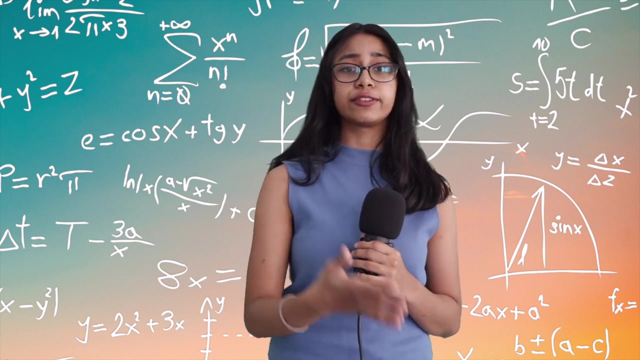 to education because they believe that it truly understand a concept, you must enjoy it. and as they focus a lot on creativity and critical thinking, they use that as the core and the essence of the learning process. for example, while teaching math- something like subtraction, addition, division of multiplication- they 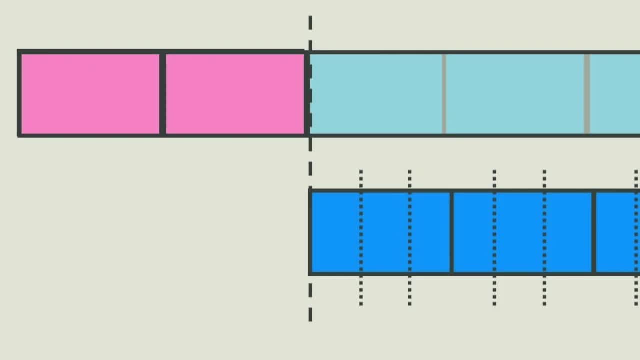 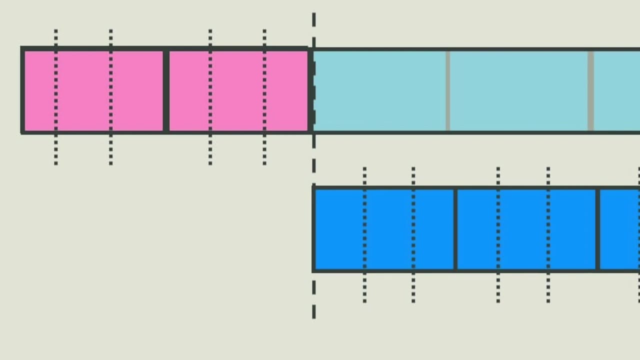 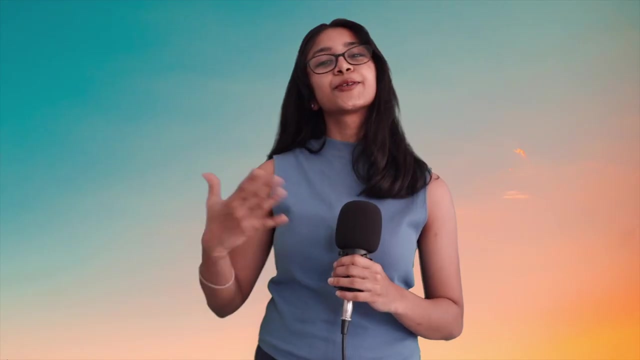 try to the famous model method. in this method, children draw a diagram with with bars and blocks in order to visualize the problem on paper. This visualization then makes it much easier for them to solve the problem in a systematic manner. Even the most complex problems can be solved using this method. Kind of cool, right. 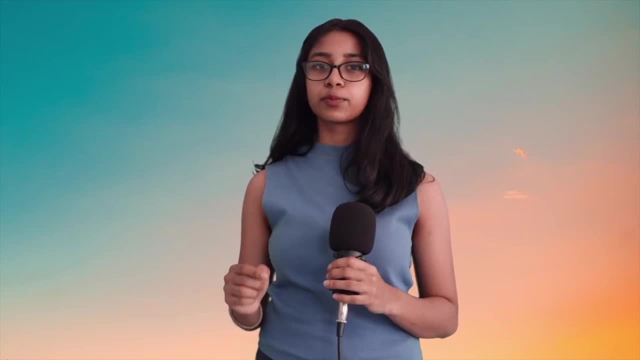 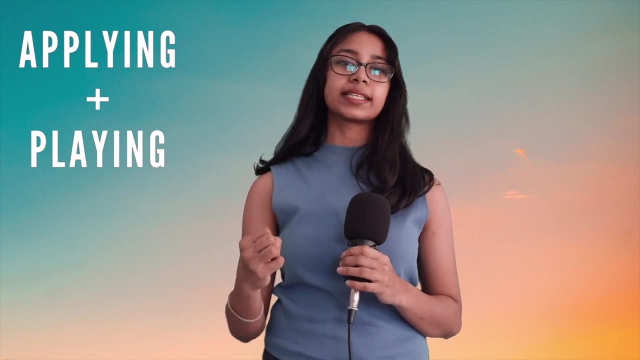 So, to give you, another example of the approach taken by schools in Singapore is that when they're trying to learn a scientific concept, they always do it by applying it or by playing with it. So this means that they're usually given a project in a pair or a team, and this 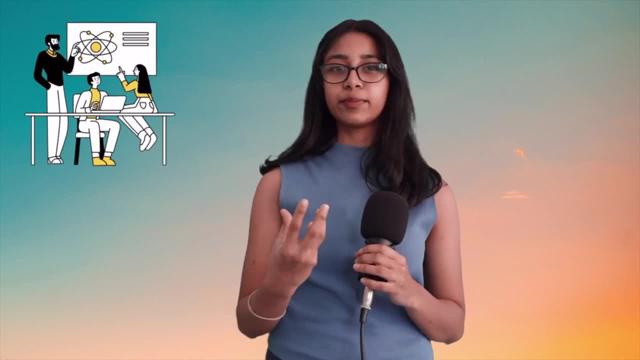 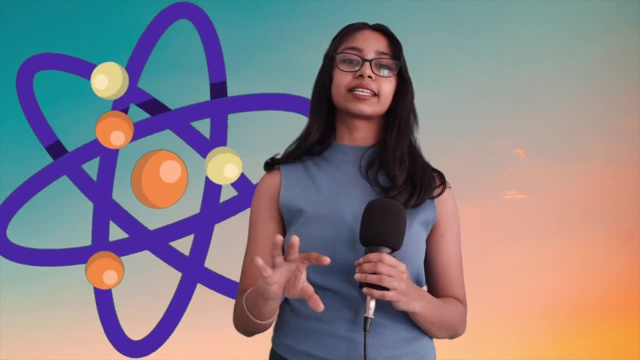 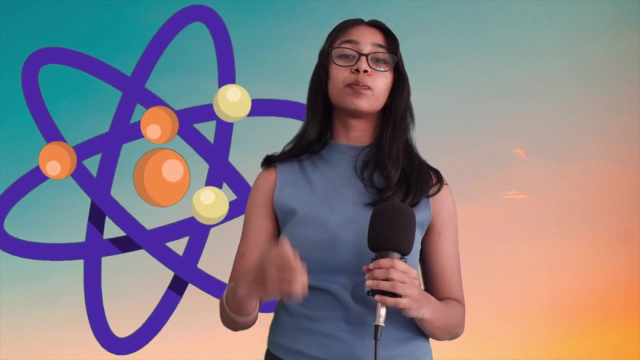 allows them not only to learn the concept in a more collaborative manner, but it also teaches them how to communicate with each other and to work as a team. So, just like maths, even science is given that playful approach, because they feel like children are already naturally curious and what the curriculum needs to do is to bring out that natural curiosity. 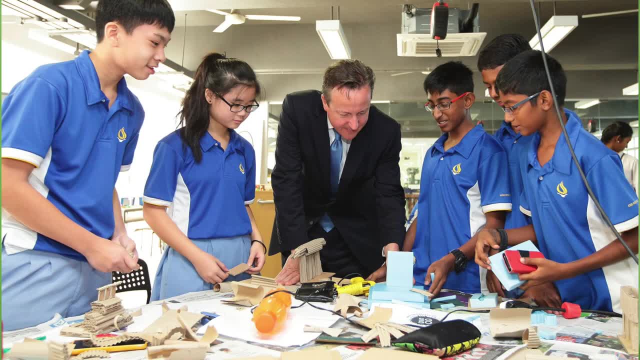 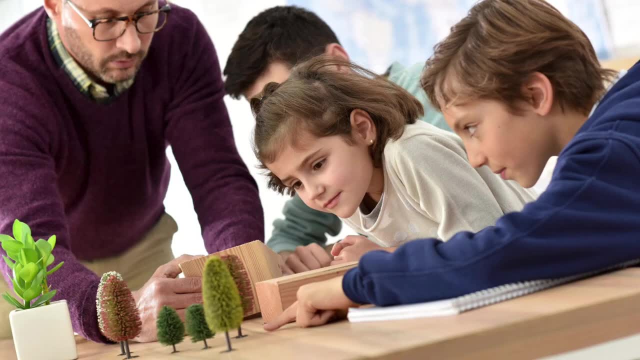 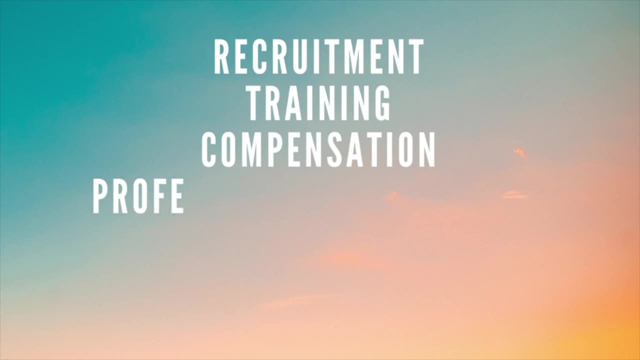 Now moving on to teachers. Singapore has a high quality teacher world workforce. The system itself makes sure only the best of the best are responsible for teaching and preparing the next generations. Recruitment, training, compensation, professional development, performance appraisal and career development: all these factors are carefully. 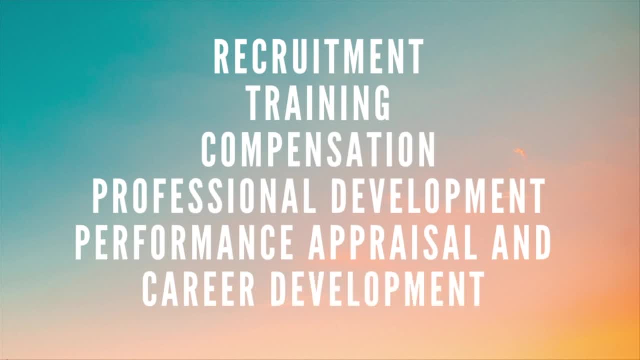 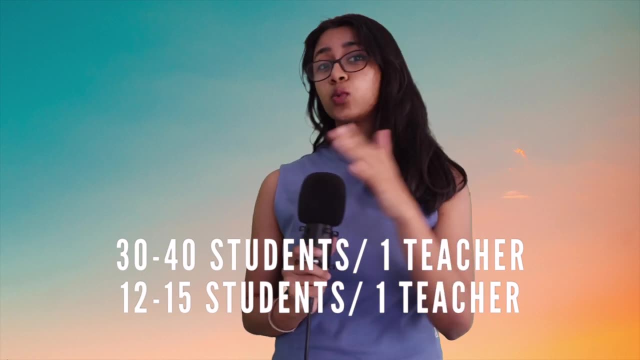 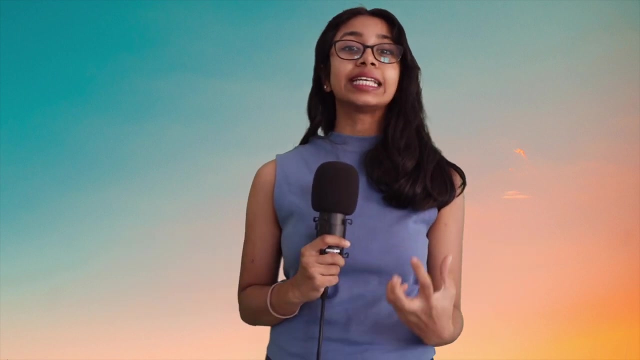 considered so that only top quality education is imparted. Also, the student ratio in India is around 30 to 40 students to 1. Whereas in Singapore it's only 12-15 students to 1 teacher. This allows the teacher to take. 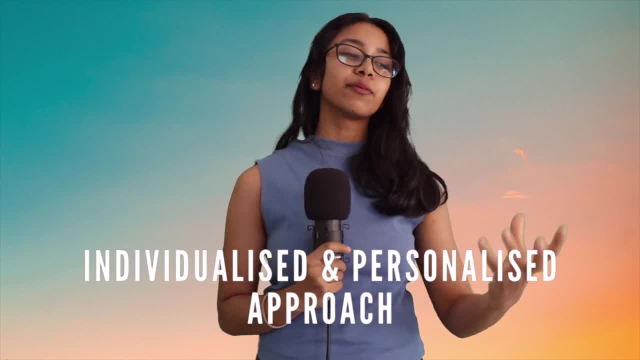 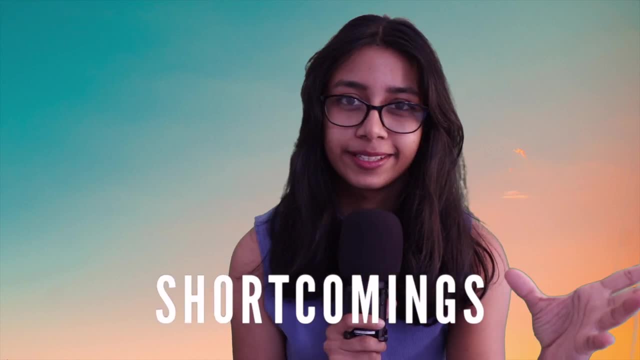 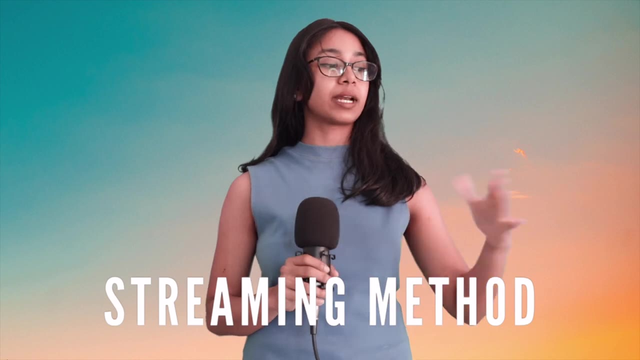 the time to understand each and every child and have a more individualized approach to education. So now let's have a look at its shortcomings. Singapore's education system follows a streaming method, meaning that from class 1 to 6 is the primary education and to go beyond that. 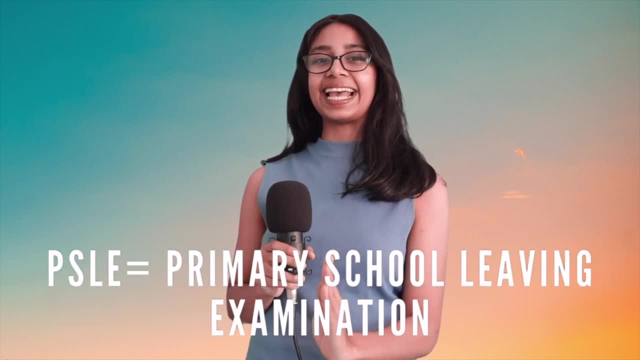 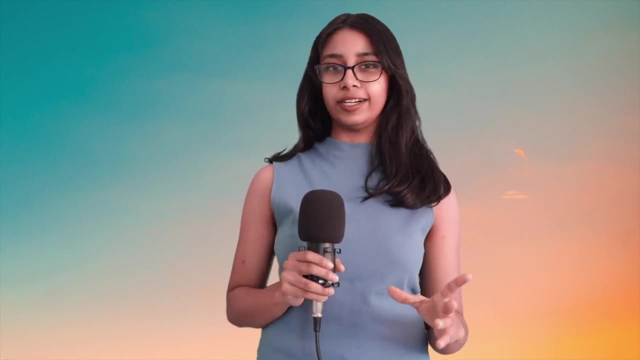 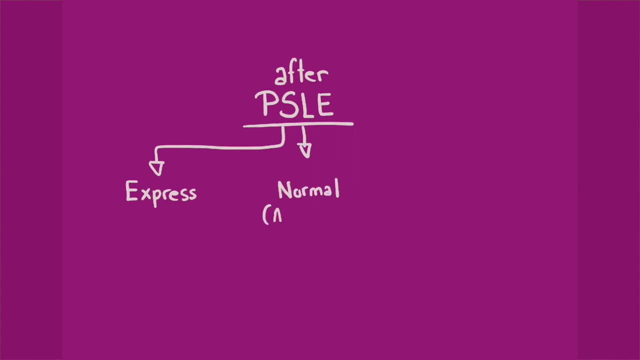 there is an examination that you need to pass, the PSLE primary school leaving examination, and it is supposed to be one of the most strenuous exams in the country because the marks that you get in that examination determines which of the three streams you get into. here are 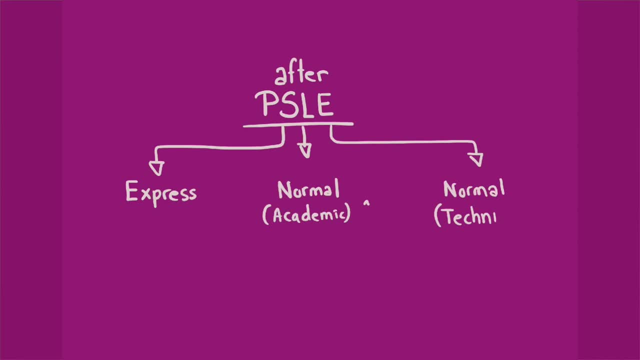 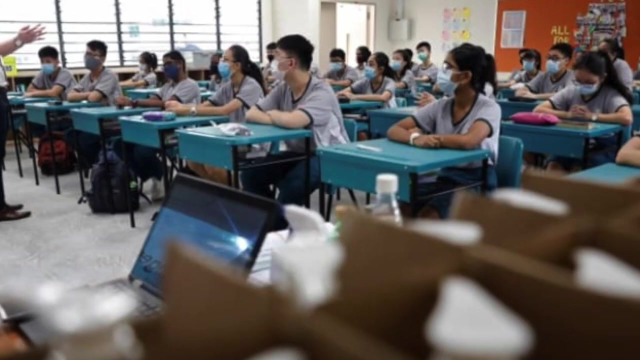 the three streams- express, normal academic and normal technical. according to their PSLE scores. you get into one of these streams, the really good students get into express, others get into the normal academic and the ones who perform the worst get into the technical. so now this becomes problematic, because the ones who get into the express stream usually 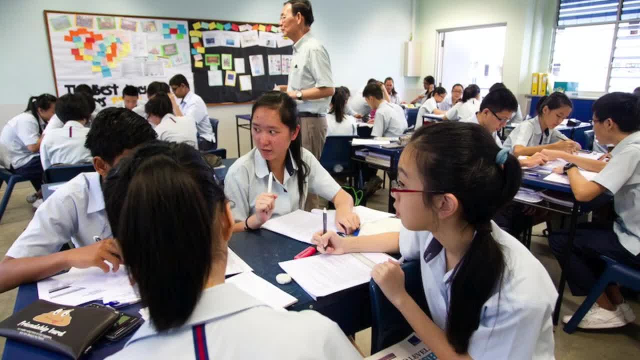 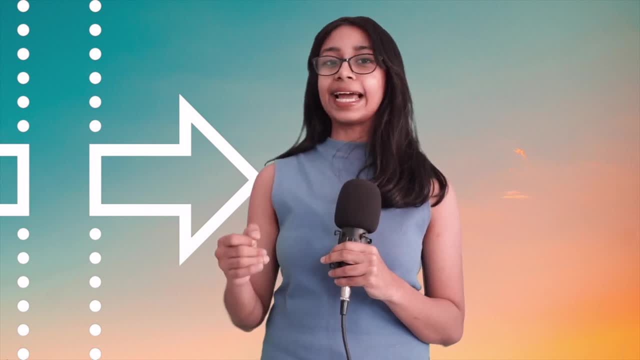 look down upon the ones that get into the technical stream. so at such a young age there is this kind of divide that is created in the students and because of that age gap between the age of six and twelve, and since this is the age that is set for the교ing age of 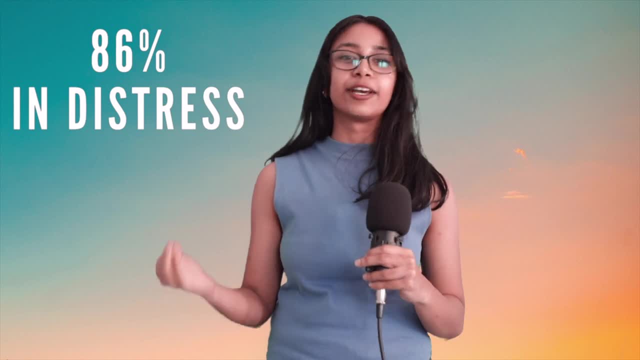 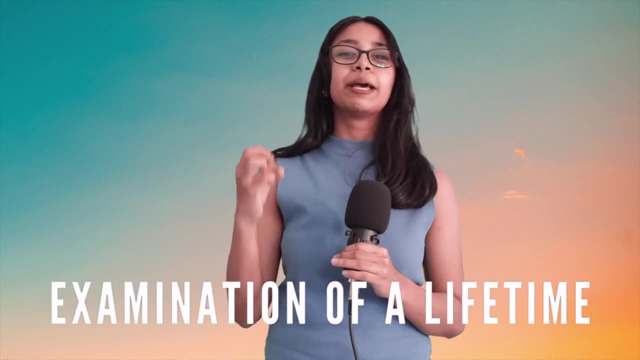 three, then you are not in the school that you should be in and it's not like you are supposed to be in, and in the school is the age that you will have to be in that age. so the parents are mainly the ones who get in the school, which has been considered as. 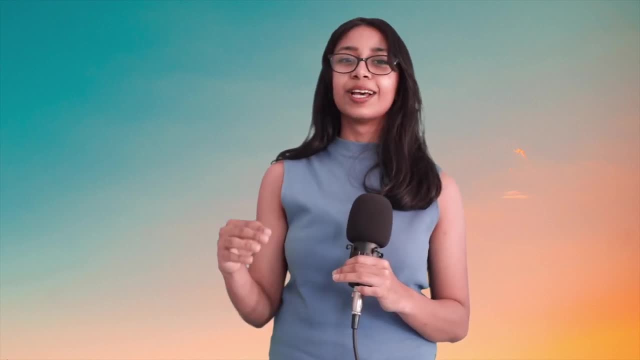 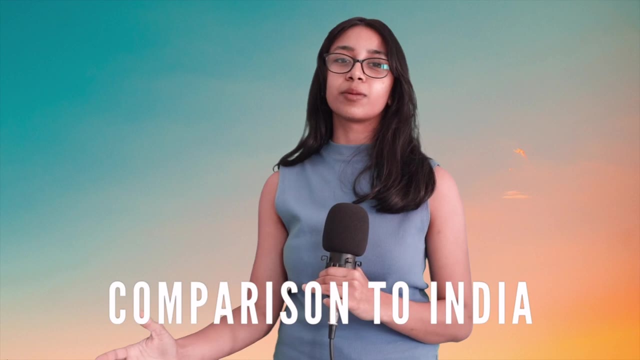 a major thing for those students, and it is known as the international exam- that the government has taken over university and they will be leaving the school and then it is time to go to university. other jobs are looked down upon, so children at that age already start. 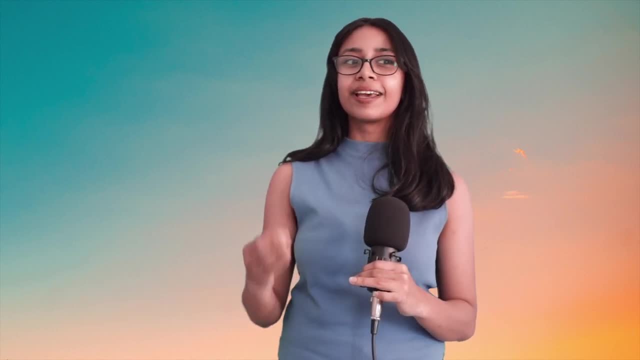 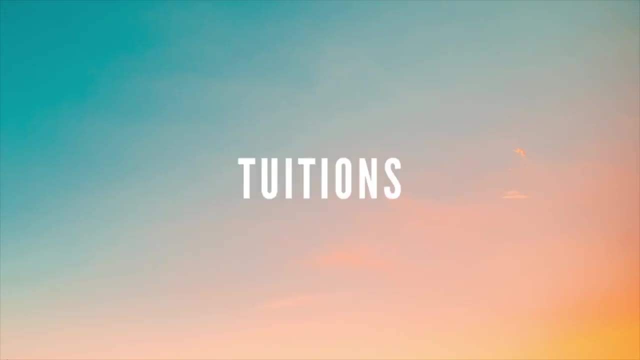 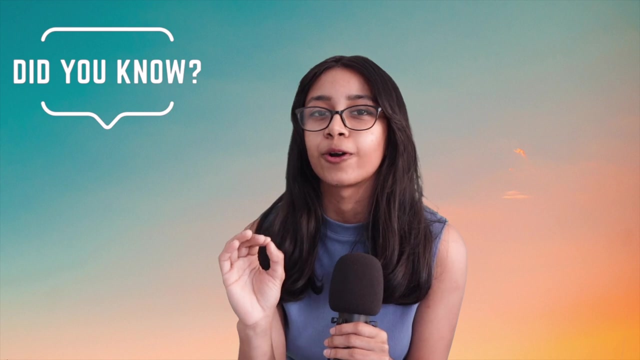 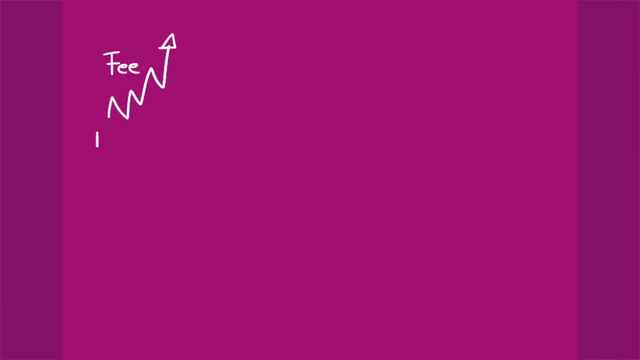 feeling this pressure and already pushed into some kind of streams, even before they get to know what they're actually into. which brings me to my next point. did you know that families in Singapore spent about 1 billion dollars annually just on tuitions? the fee increases as the child's age increases, and it is at 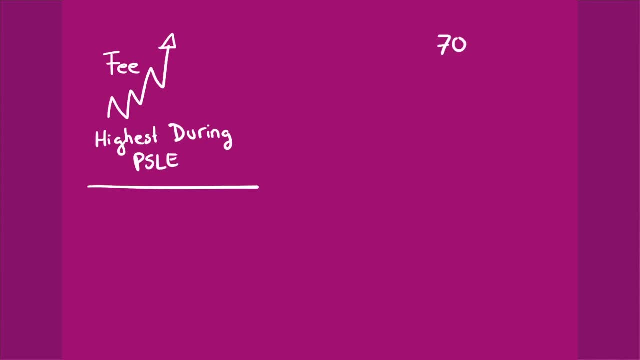 the highest when they get closer to the PSLE examination. almost 70% of elementary school children attend tuition. yes, 70%. and what is even shocking is that 40% of the kindergarten children also attend these tuitions, so children as young as 5 years old. 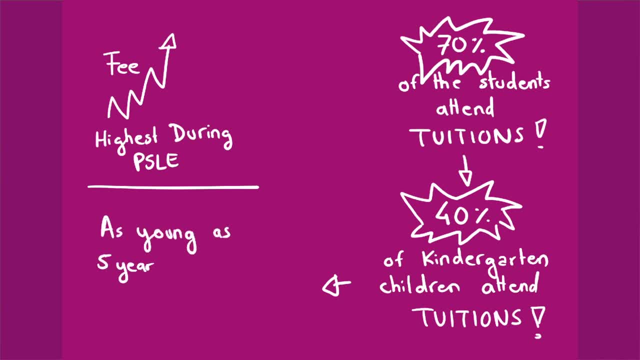 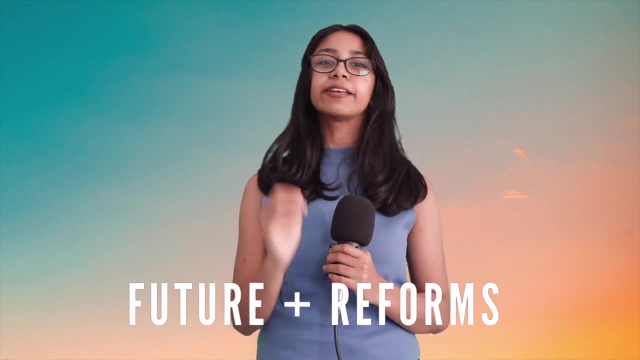 spend hours and hours in these tuition centers after school, when they could actually be spending the same amount of hours pursuing interests and passions, or even just playing. Now let's talk about the future of Singapore's education system and the reforms that they're going to bring. 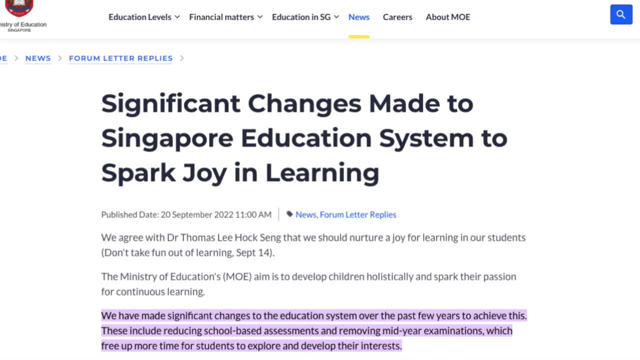 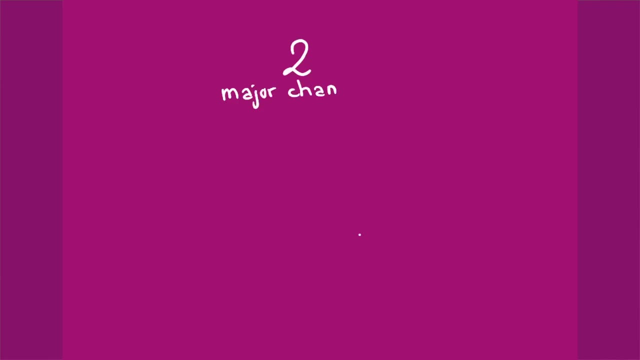 So recently, the Ministry of Education in Singapore has been thinking about reforms that would actually bring back the joy of learning in each and every student in the country. Here are the two major changes that have been, and are going to be implemented. Number one: removal of mid-year examinations. There are no more mid-year exams in primary and secondary. 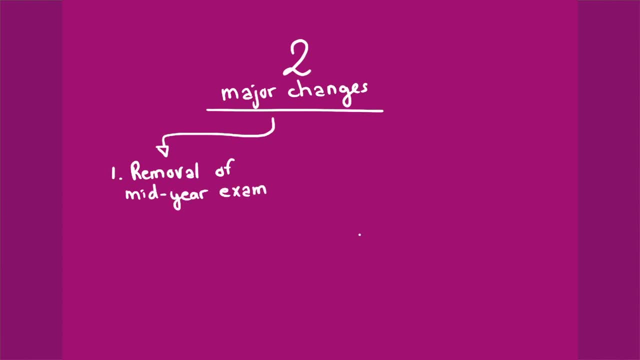 schools. This comes as a huge relief to not just children, but also their parents and teachers. So, instead of preparing for exams in order to just get a grade, children now have the environment to choose: environment and time to develop a love for learning. 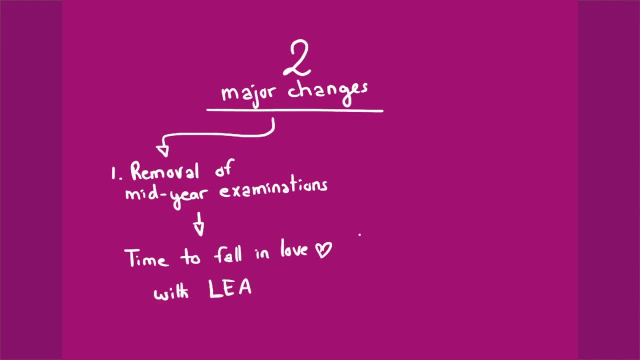 At number 2, there is abolishment of streaming. I mentioned earlier about how students were divided into 3 courses: right express, normal academic and normal technical. This is going to be replaced by a full subject based banding. Now what does that mean? It means that now. 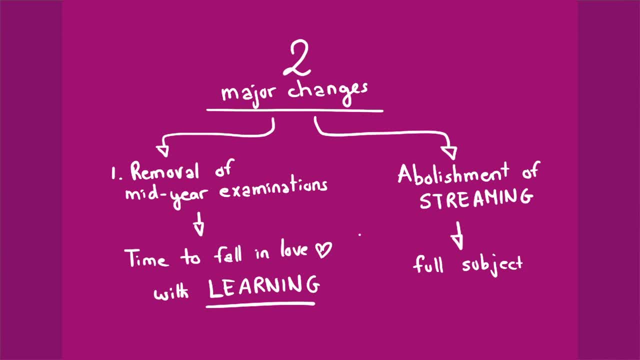 students will not be divided into streams like earlier. instead of that, they will be in mixed form classes, So students will be able to choose the subjects they want to study and are interested in. It is estimated that by 2024, full subject based banding will be: 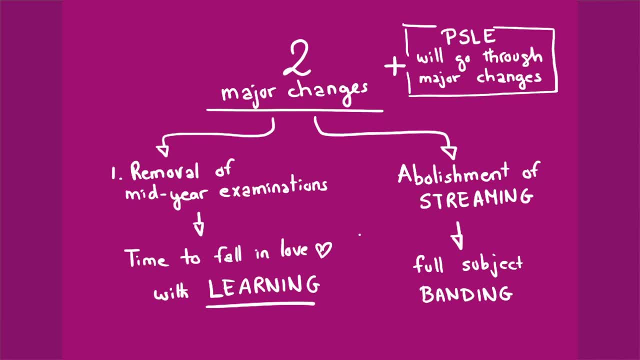 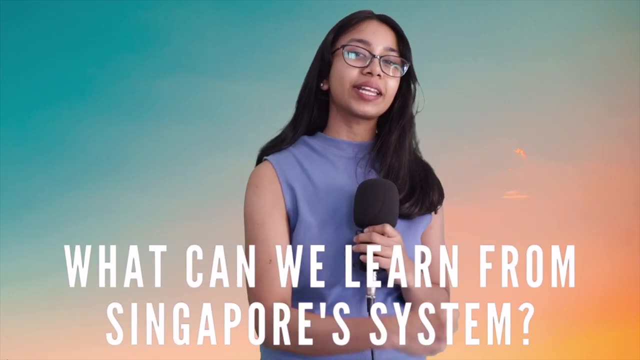 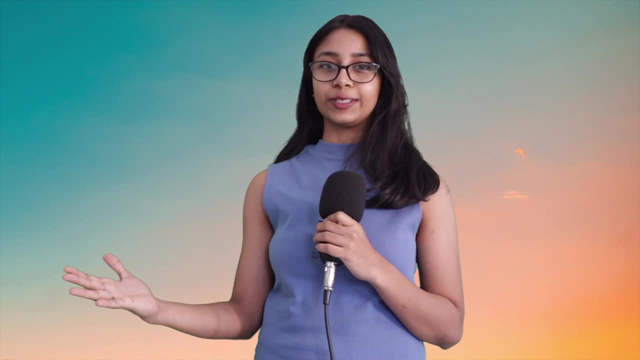 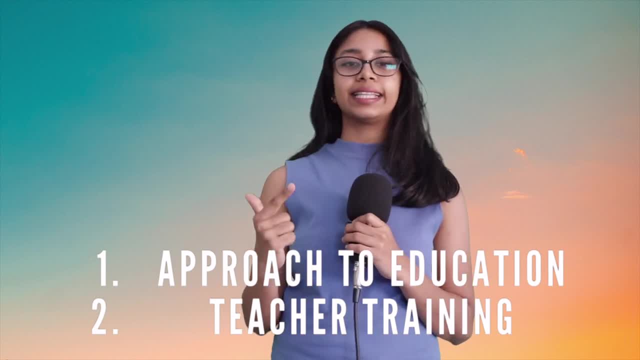 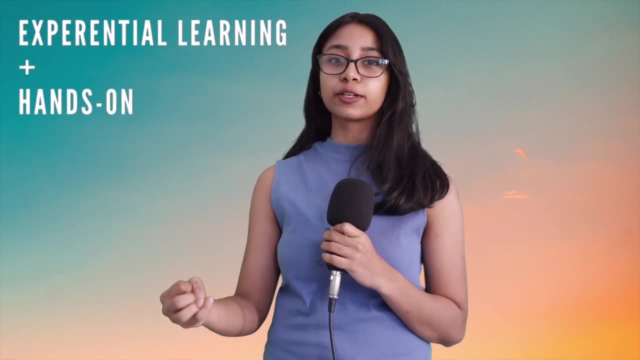 1 is their approach to education and number 2 is their teacher training. We need to start focusing, as a country, on hands-on experiential learning, just like Singapore, so that we not only allow the children to fall in love with learning and understand the concepts better. 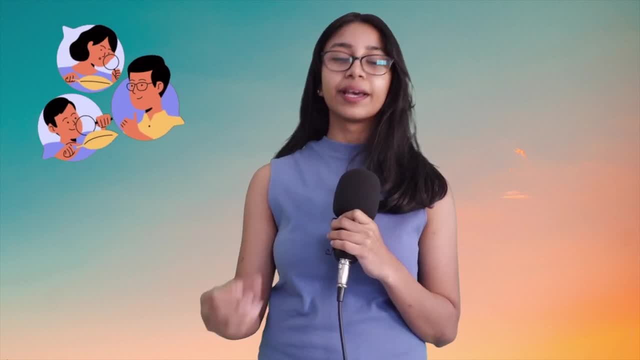 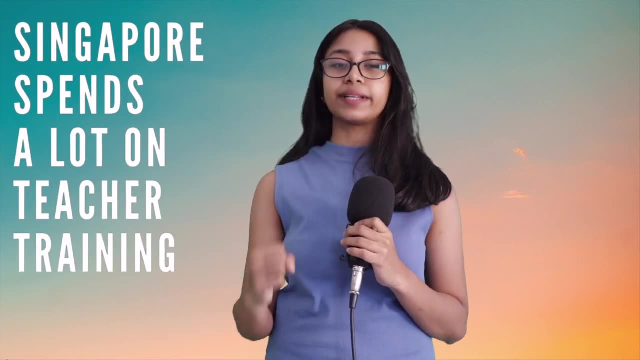 but they're also ready for everything that life is going to throw at them and they'll them, and also be ready for the future of work. on the other hand, teacher training is something that the singapore government spends a lot of time and money in, because they feel like, if you have, 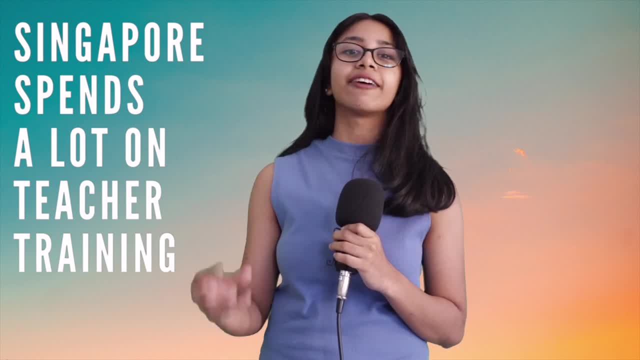 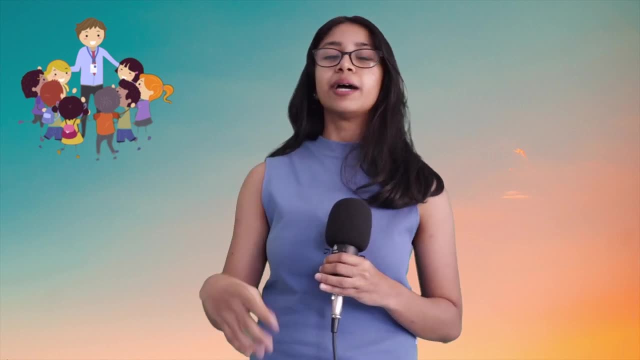 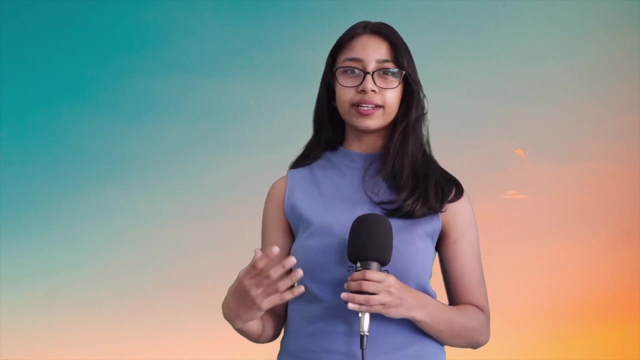 quality teachers, you automatically will have quality education. so as a country, we can really start focusing on teacher training, and not only training them professionally but also giving them that safe space to express and giving them a space where they feel respected and supported. so i feel like if we can draw a balance between the approach to education which is more experiential,